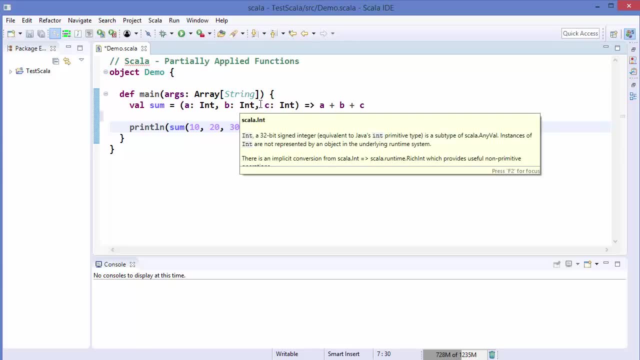 three arguments and you are set to be applying that function, so this code, to these three arguments. And when you use this function like this, so you use the name of the function and then pass all three arguments. this kind of functions are called fully applied. 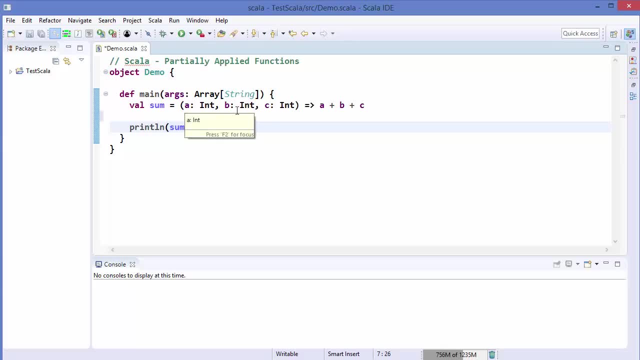 function, That means you have applied all the arguments to the function. So this is called fully applied function. Now, what is a partially applied function? So in the same example, for example, you just provide few arguments. Let's say you provide just two arguments and 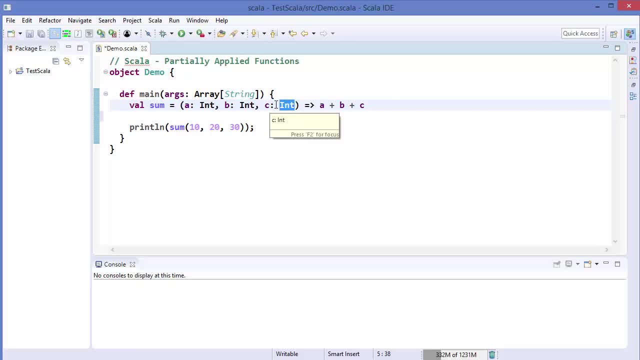 third, you keep it as a default or a wildcard, some kind of a wildcard. then it's called a partially applied function. So let's see how we can use partially applied functions in Scala. So this is the normal usage of this sum function. You just declare this function sum function and then you call this function with all three arguments, right. 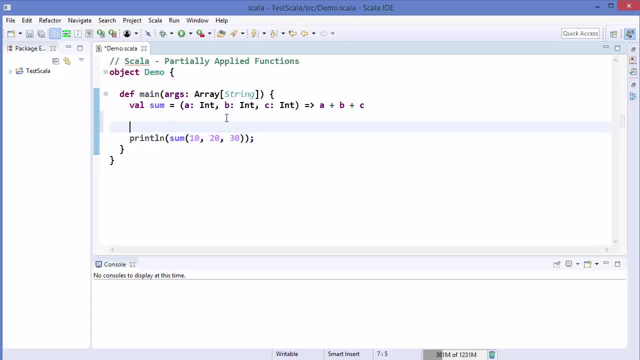 Now what I do in between here is I will declare one more function and let's say this function name is f, and then I just call this sum function and then I just pass for example 10 as a first argument and then 20 as a second argument, and 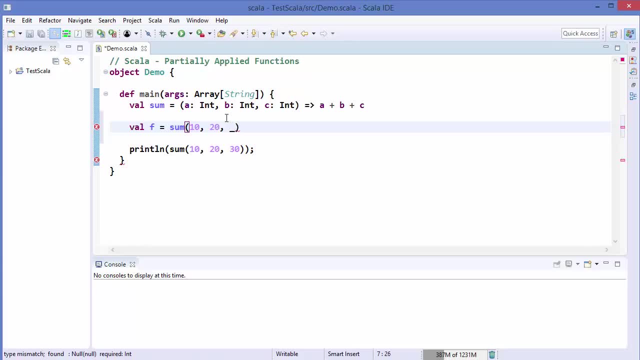 the third argument, I am going to keep it as a wildcard. In the last video we have seen that we can use underscore as a wildcard, right? So just write underscore and then colon and then data type of that argument. okay, So what we have done is we have fixed first two arguments here and the third argument. 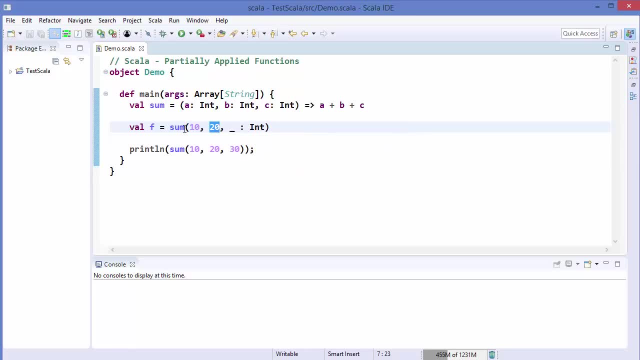 we said that we will just pass it whenever we call this f function. Okay, So now what we can do here is we can call f function instead of sum and because we have already passed first two arguments in the sum function, when you just pass. 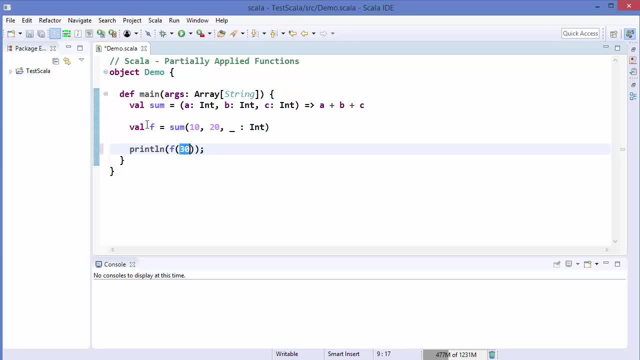 30 in the F function, then it will be applied to this wildcard. okay, so let's save the code and run it and let's see what's the result of this function. and you can see: the result is 60. so first, two arguments here are fixed, and the 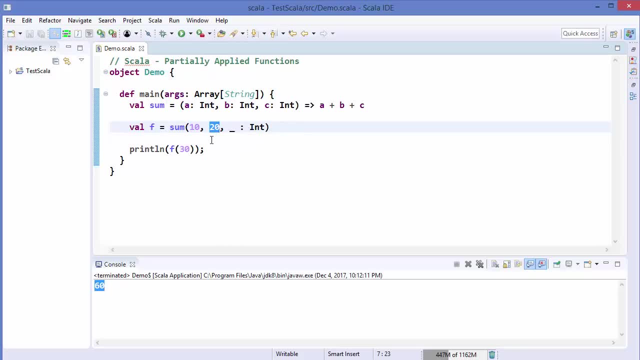 third argument: we are considering it as a wildcard. so this: whatever number we will pass here- for example, I pass 100 here- it will be applied to this sum function and then it will show the result in a similar way. if you want to just apply one argument and past two arguments as wildcard, you can just write: 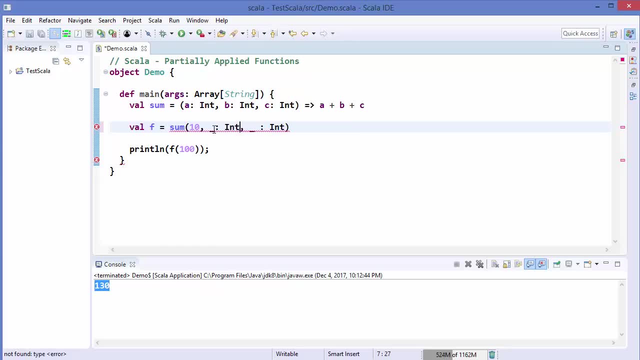 underscore colon and then int for the second argument also, and then you can just pass two argument for the F function, so hundred and let's say two hundred- we passed two arguments here- and then run the program and it gives us 310, which is the sum of this, this and this. 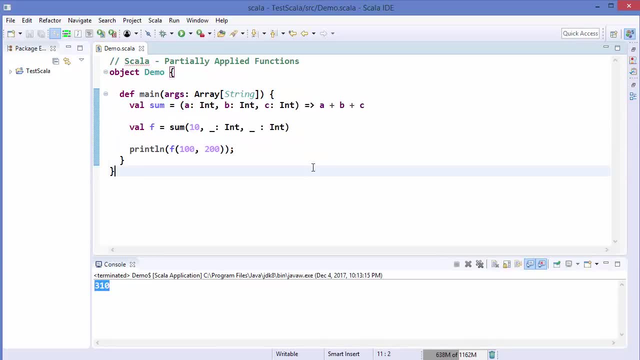 and this is called partially applied function. now, this was a very simple example. now let's say in a real world example: you want to log something, so let's define one another function here above the main method. so I'm going to define def log and what we want to do here is we want to log. 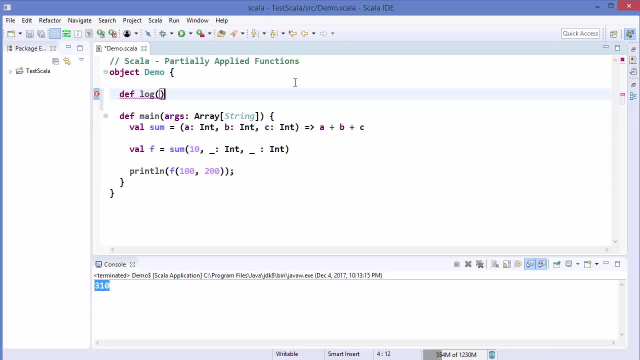 something now, right. so log function generally. we use to log some messages in some situations. so, for example, if your code throws some error, we want to log something and we want to know at which time this log is created, right? or if you want to show some information. 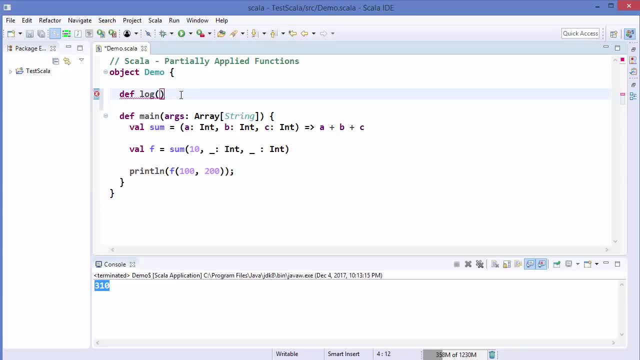 to the user of the code, then we use log. or in the case of warnings or some critical condition is happening in your code, then you can use a log function, right? so what are the argument we want to pass in the log function? so the first argument we want to pass is the date. so we want to print. 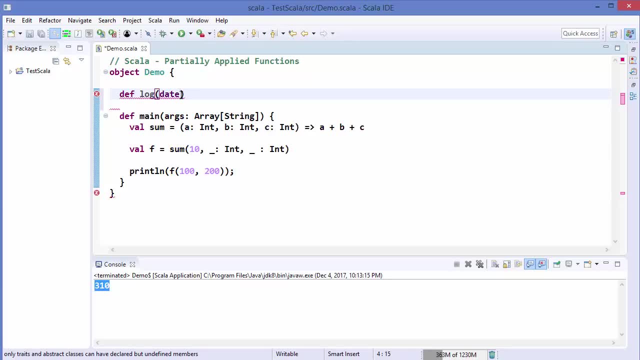 the date and time at which this log is created. and the second argument we will be the message. it's ready to be sent in. so that's the first. that's the whole argument. basically. in that case now to use date, we need to import the date library. so just write: import java dot util dot date. okay. 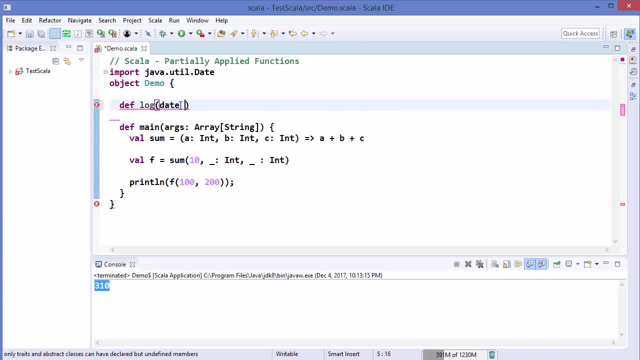 this is going to import the date library, and here the data type of date will be date, and the second argument here will be a message, let's say, and the data type of message will be the string. and what it does? it just prints this log message. okay, so what we want to write here is print L, n and then. 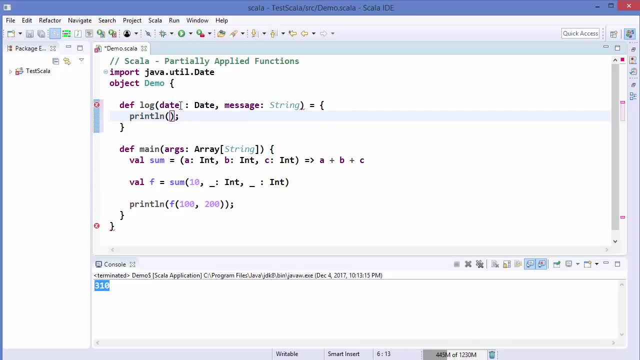 we want to just first of all print the date first of all and then plus, and let's give some space between date and message and then plus message. okay, so what it does is this log function: just print the date first of all and you then prints the message. so now let's create a partial function out of this log function. okay. 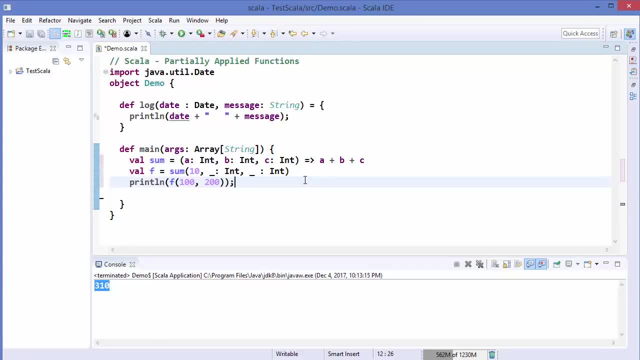 so what we want to pass into this log function? first of all we want to pass the date, so we can just define date first of all, and then we will write new date which is going to give us the date, and then we will just define a new variable. let's say the new variable name is well. 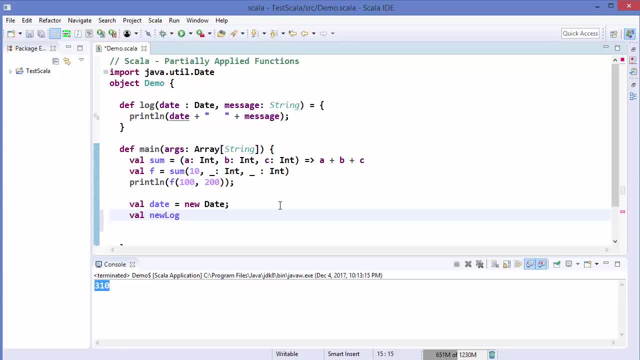 new log. okay, so new log is our new function. let's say: and then we are going to apply a log function here, so log, and then we will apply date here first of all, and the second argument will be partially applied. so underscore, colon, string. okay, so what we want to do is we want to apply a new date and then we will just define a new date. 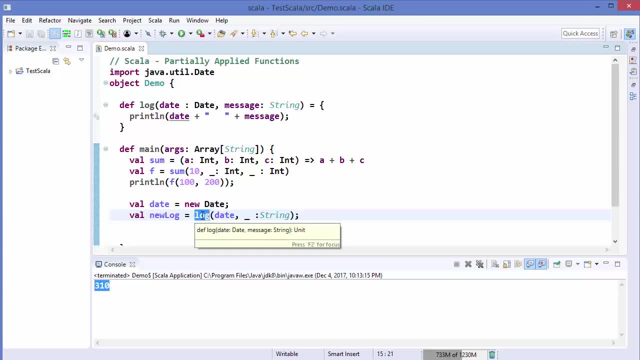 we have done. we have created a new function, new log, and then we have just assigned this log to this new log, and we have already applied one argument to the log function, but the second argument is the wild card here. okay, so now what we can do here is we can call new log. 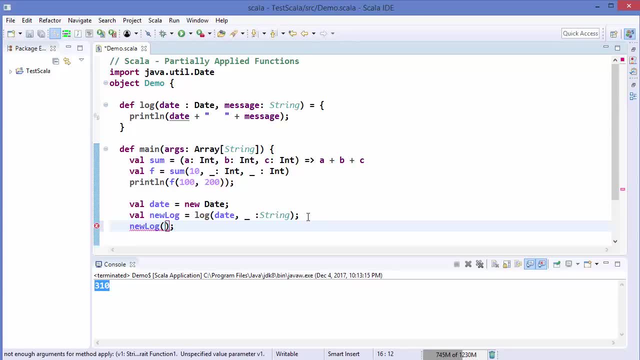 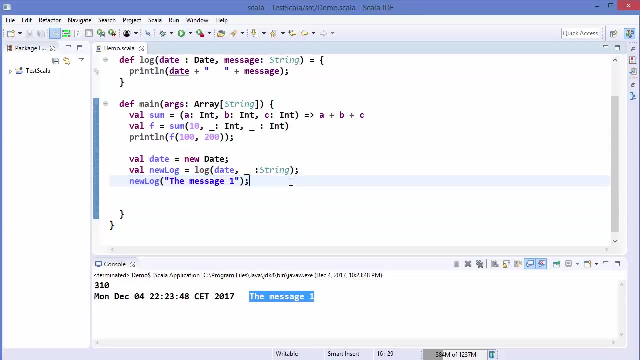 and then we can just give our message, for example. so let's say message one, let's say okay, and then let's run the code and it's going to print first of all the date and time and then our message. now we can call this new log message multiple times like this, and let's say message: